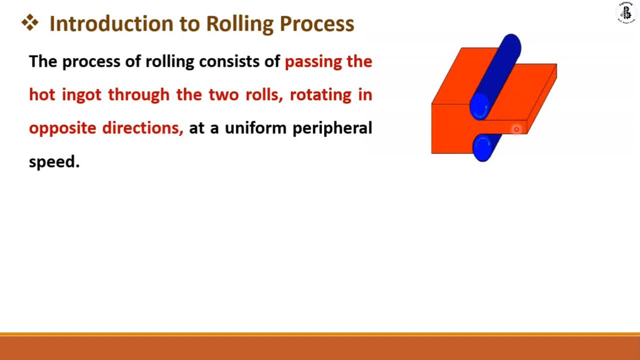 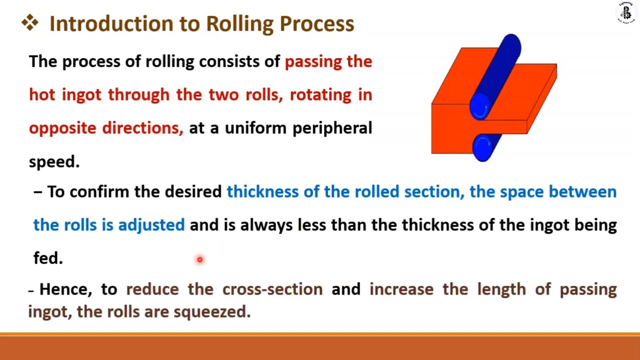 cross-sectional area and increasing into the length. so in case of the rolling that is, the make or conformations so desired thickness of the roll sections, the space between the roller is being adjusted according to my requirement of the thickness as well as the cross-sectional area. so in case of the rolling process we already discussing there, reduce the cross-sectional area. 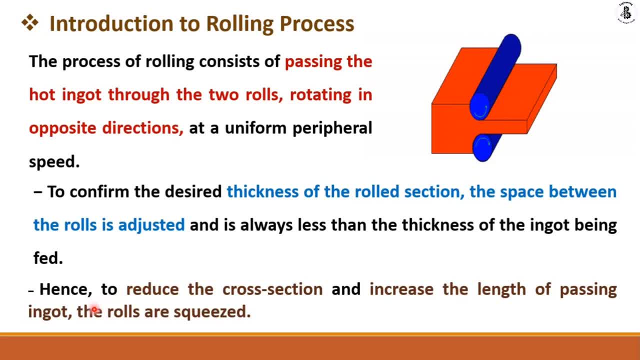 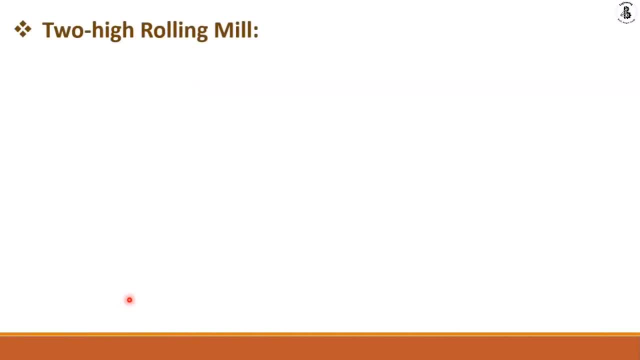 and increasing the length of the passing of the ingots, the rollers are squeezed. so, according to the requirement of the different shape and size, i would like to select different rolling mills, starting with the first one, two high rolling mills. so just you can see two high rolling. 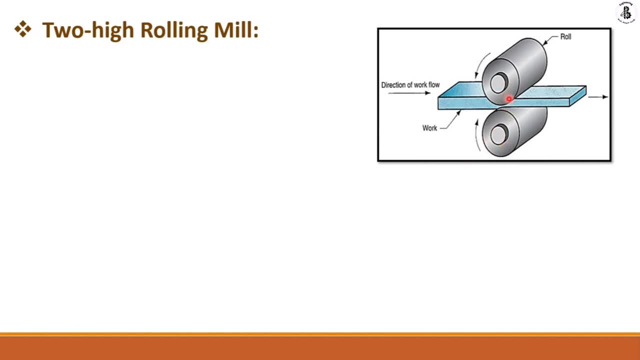 mills are being used and, according to that name, two pressurized roller is being used to converting my raw material into desired shape and size. so one of the end that will be the direction of the workflow and another end that will be my product. so, in that case, of the two high rolling mills, both 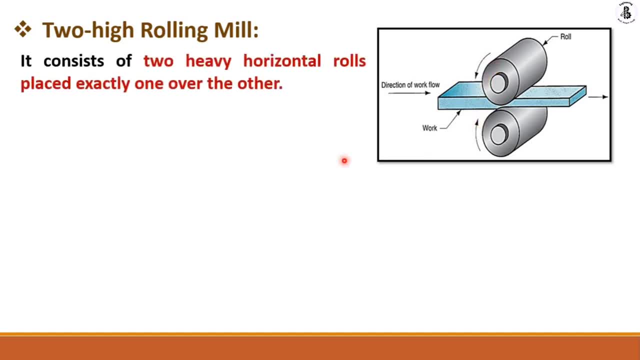 the rollers are rotating into opposite directions. that will be considering as a two heavy horizontal rolls place exactly one over the another. that is the main requirements. the space between the two rolls can be adjusted by rising, or you can say the lowering, the upper rollers, whereas the positions of the lower roll is fixed, so lower roll. 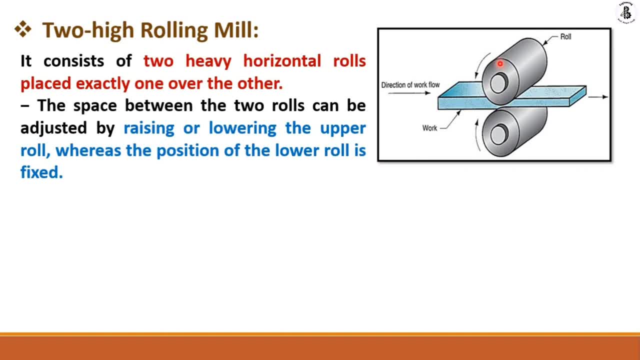 is being fixed. upper roll is being movable. so, according to my requirement of the cross-sectional area, i would like to adjusting the center distance of these two rollers. both the rollers rotate into the opposite directions that we already discussed. in this type, their direction of the rotation is: 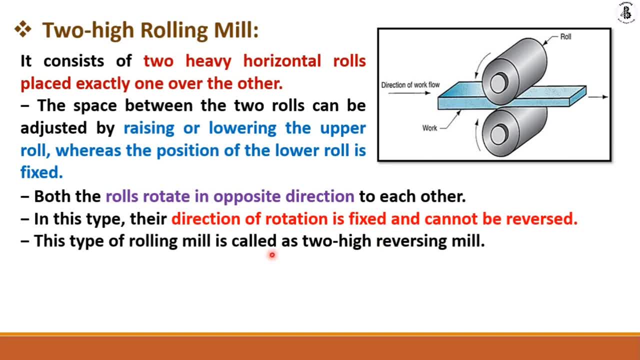 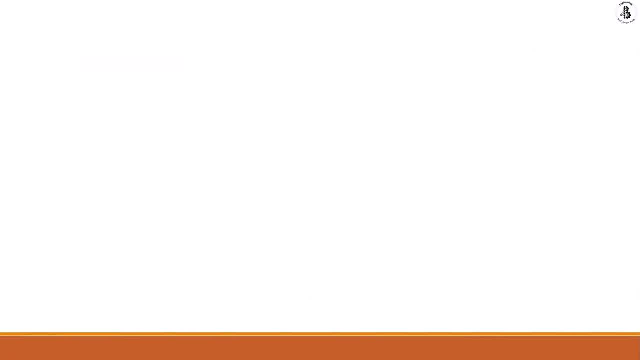 fixed and cannot be reversed. this kind of rolling mill is called as a too high repulsing mills. second one, according to my shape and size, will use three high rolling mills. so just you can see the figure. so according to that name, three rolls is being used to converting our raw material into desired shape and size. so if you 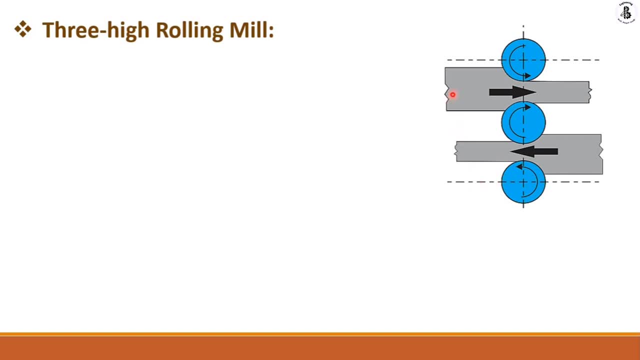 want to reducing the high amount of cross-sectional area of your raw materials. so either you can use the multiple plus, you can use the three roll mills. so this is the end of the introducing of the rowing mills materials. so there is my first pass. so in that case it will be contacting with the one and two. 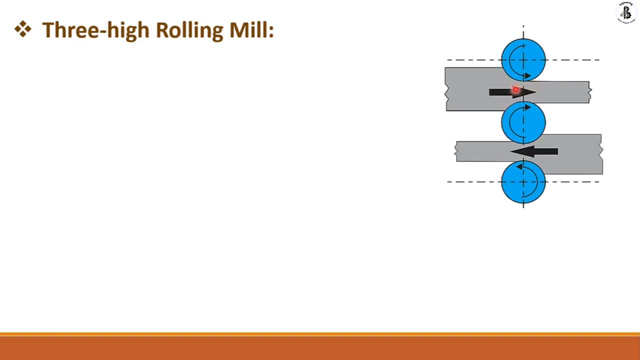 and after it will be completing the total movement from one end to another end. once again it will be from the reverse side. so from one cycle the amount of reduction of the cross-sectional area of the more as compared to two high roll milling process. so just you can see. 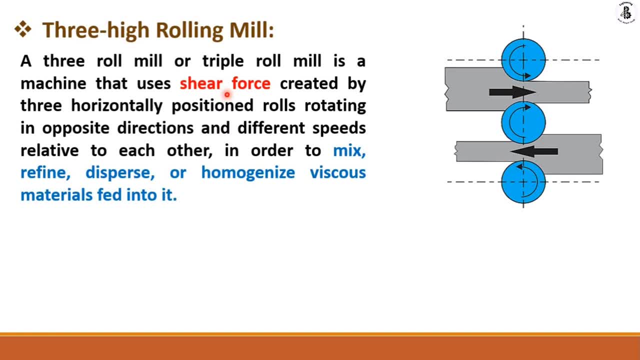 the three roll mills, or you can say triple roll mill, is a machine that, using shear force that will be created by the three horizontal positions, roles rotating in opposite directions and that will be having a different speed relative to each other. so in order to mix, refine, disperse, or you can say: 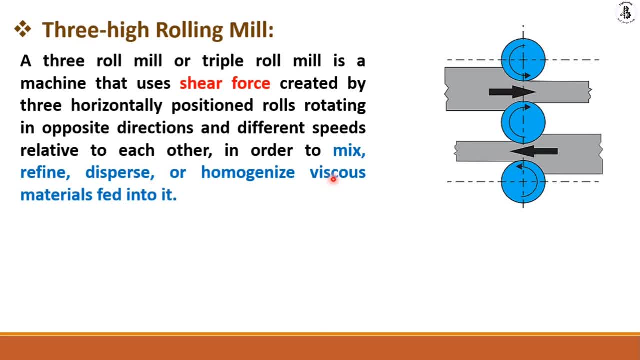 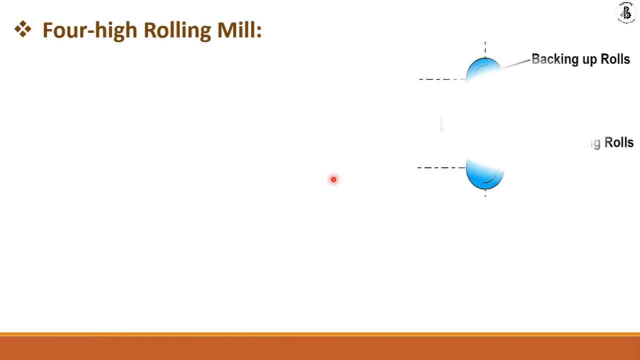 homogeneous, viscous material pad into it. so, according to my requirements, i would like to select two or three rolls mills, three high rolling mills, third category of the rolling mills, and that will be four high rolling mills. so just you can see the structure. so, in that case, of the four high rolling mills. 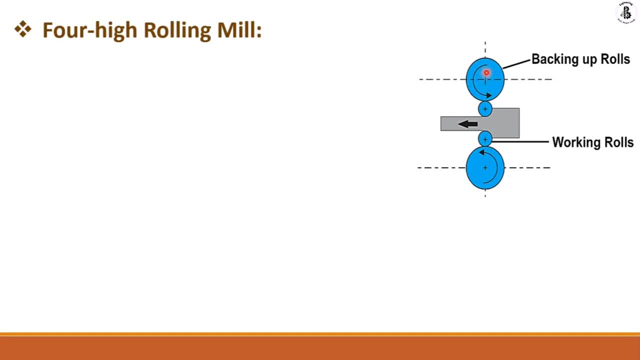 two main backup roles are being used and just you can see into the figure two small diameter roles and that will be considering as a working rules. so these working roles, it will be directly contact with the workpiece material and one of the periphery of that working roles it will be. 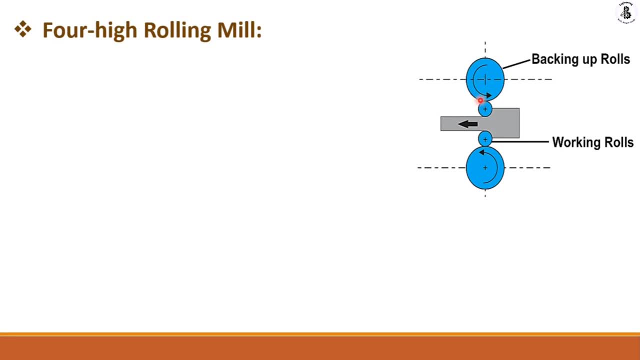 contacted with the backing of the rollers. so if you want to work onto the harder material converting into desired shape and size, so basically that kind of extra stress is being developing with the help of these working roles. so in that case it consists of the four horizontal roles that we already discussing. 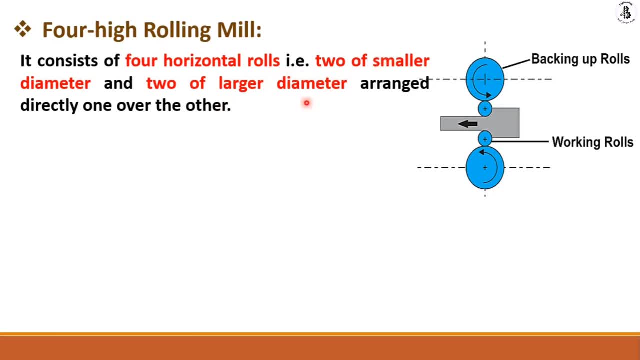 two smaller diameter and two larger diameter arrange. it will be like that and after that the larger diameter rules are to be said as a backup rolls and there has been used to prevent deflection of the smaller rolls, which otherwise would result into thickening of the roll plates or seats at the 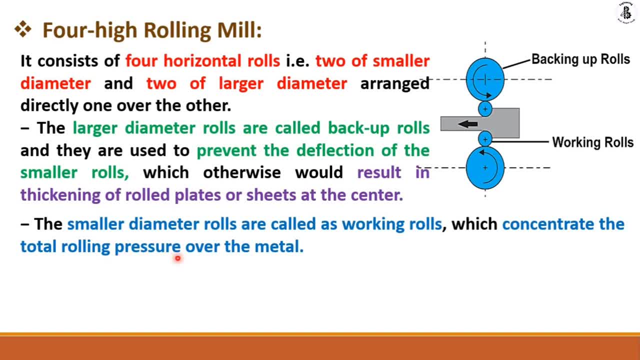 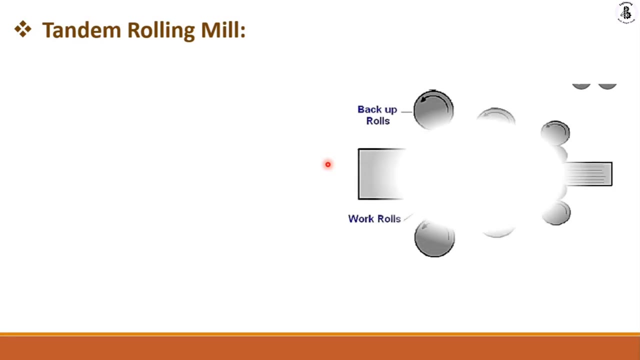 center. basically the small diameter rolls are called as a working roles and with concentration, the total rolling process over the metal. the common product of these mills are hot or cold rolled sheets and you can say plates after tandem rolling mills. so just you can see the figure. so in that case of the tandem rolling mill, just you. 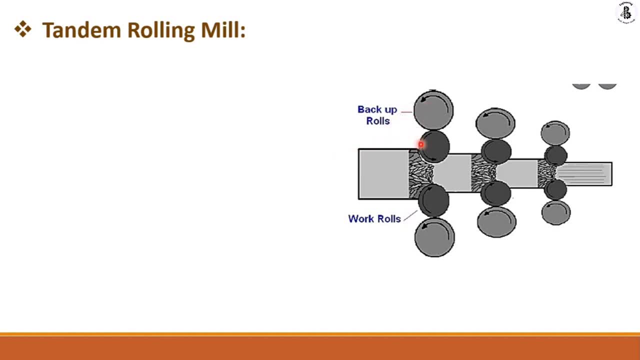 can see the number of backup rollers along with the working rollers and just you can observing that the work is that will be fed at the one of the end of these kinds of tandem rolling mills and it will be having a large amount of reduction into cross-sectional area, into single pass. so in case of the four roll, 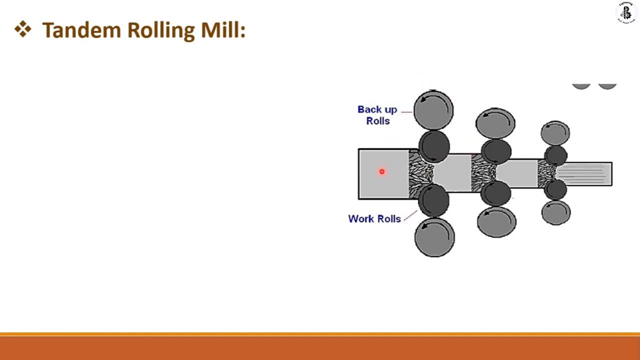 mills that will be having a high efficiency, as well as the reduction into time to converting this raw material into finished product. so in case of that set of tools, or three stands roll set into the parallel alignment so this facilitate a continuous pass through the each one successively without change of the 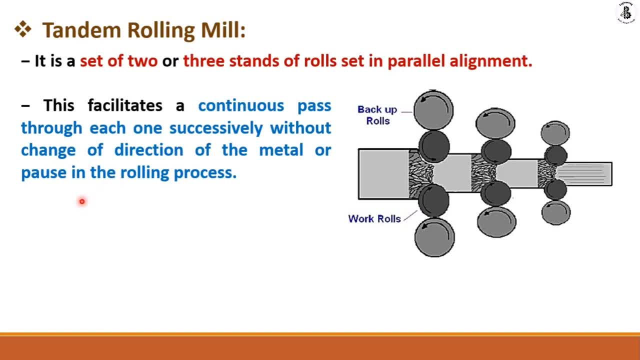 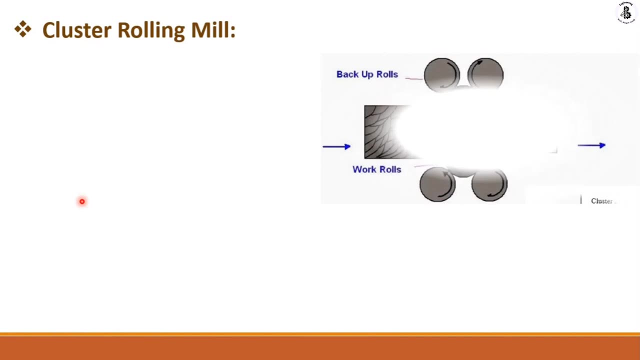 directions of the metal opposed in rolling process. so that will be reducing the manufacturing time basically, and that is also increasing the productivity of the product after this cluster rolling mill. so just you can see the figure here. that will be the one side to backup roles and a single working roles. 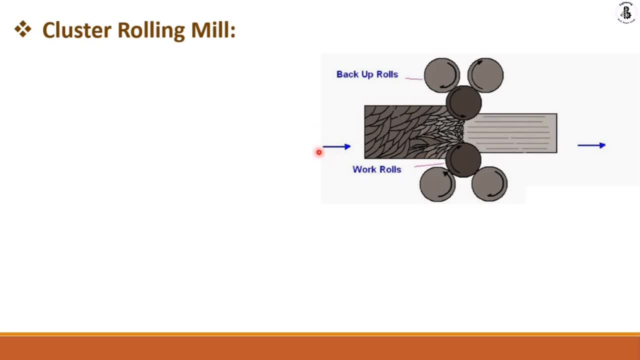 so as from the rolling process the workpiece fade at the one of the side and converting into desired cross-sectional area. so in case of the cluster rolling mills it will be considering as a four high rolling mills, so which is considering as a special kind of rolling. 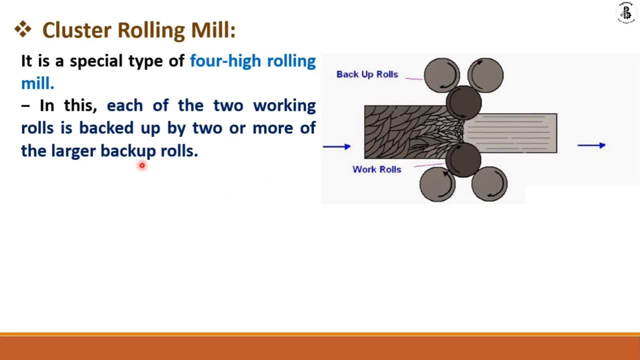 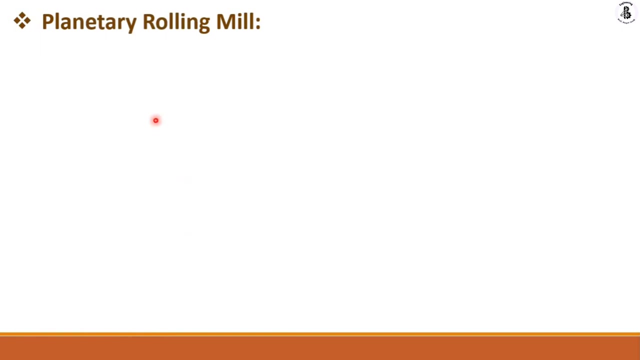 process. so in this each of the two working roles is backup by two or more of the large backup roles for rolling process, the hard, thin materials it is necessary to employee work roles of the very small diameter but of the considerable length is a normal rules being at it and one by one, each role's it will be having a content. run a process, been a running machine. you can see that from the feet orutes, from 1, 2, 3, 2, J자 і figres. moments around this backup roles there are number of small size of the roles is being a taste and one by one, each rolls, it will be having a contact from upper side. also, crushed means around these backup roles there are number of small size of the rules is being a test and one by one, each roles, it will be having a contact equal angeatres partner. 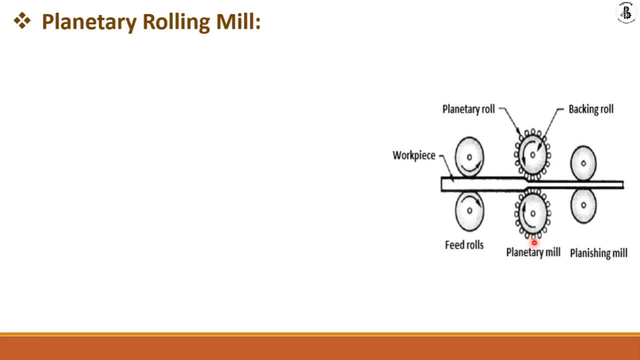 as well as from the lower side. so just you can see, it will be the one kind of simple rolling process, but these backup rolls and that will be having a number of planetary rolls, it will be attached. so at a time there is a two or three rolls is being in contact from the upper side as well as. 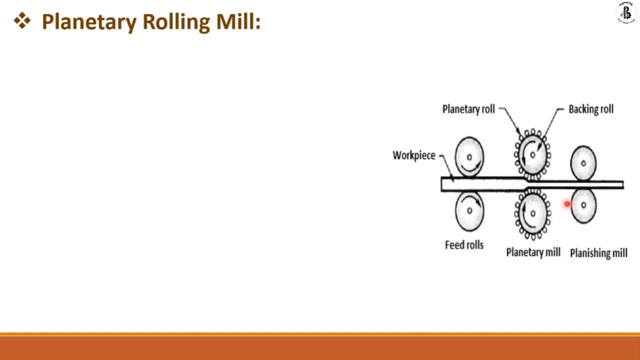 from the lower side and finally it will be the planishing mills. so in that case the different kind of rolls is being used: first, these feed rolls that will be only used to feed the workpiece material, and these planetary mills that will be used to decreasing the cross-sectional area of the 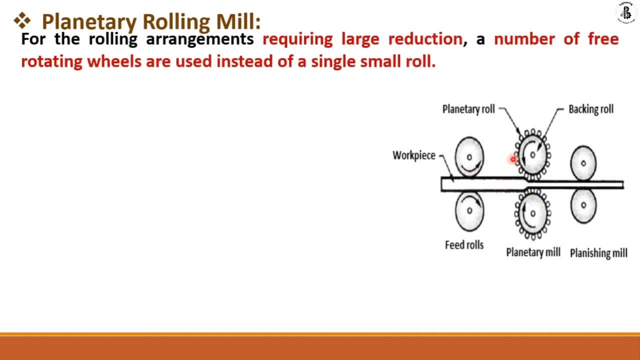 workpiece material. so in case of this planetary, the four rolling arrangement requiring the large reduction of the cross-sectional area and a number of free rotating wheels are used instead of the single small roller. so this kind of planetary rolling mills that will be having a high efficiency as compared to other.